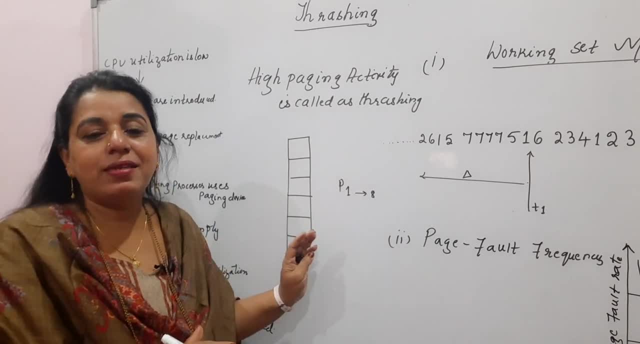 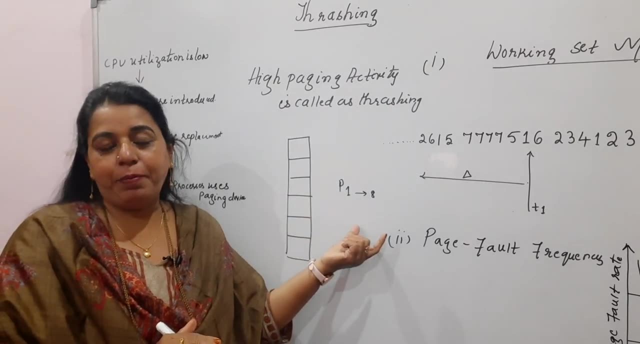 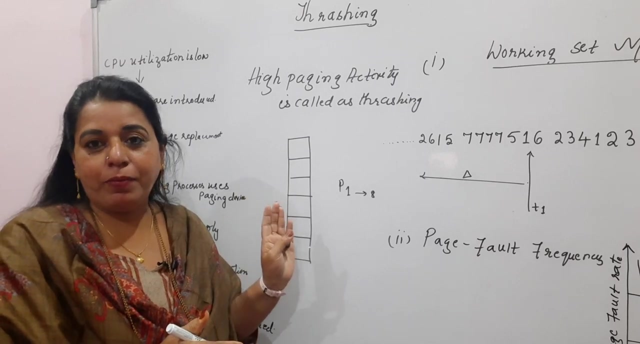 way the memory itself will assume to be very small in size. it has got only six frames and those six frames are allotted to the process p1. So p1 actually has got eight pages. but getting six pages is also what for p1. most of its contents are there in the main memory. So 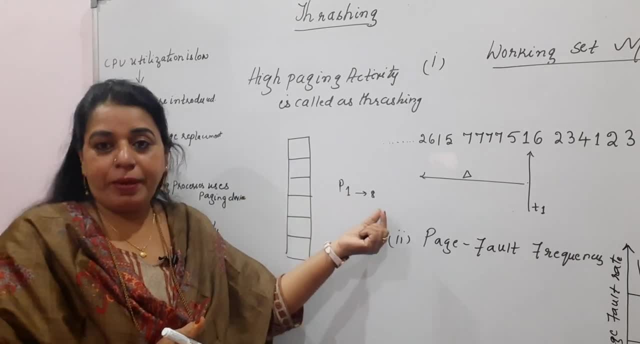 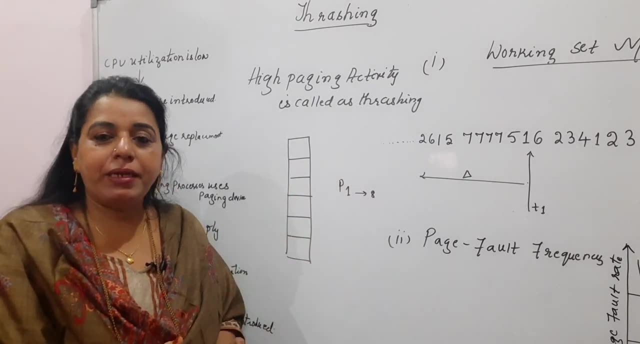 the execution goes on smoothly, Then the other two pages. whenever it is in demand, definitely those pages will be replaced with any of the two pages, depending on the what page page replacement algorithm is used. So fine, so we can say that, yes, the page fault is minimum here. 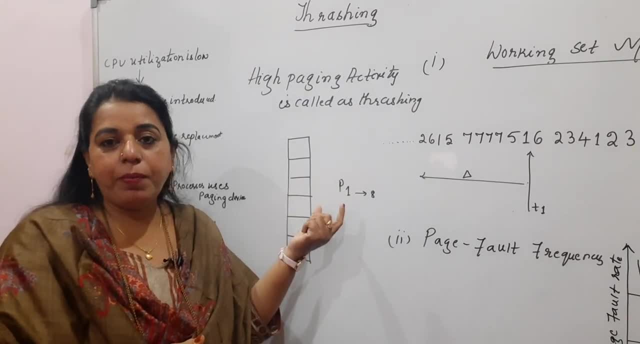 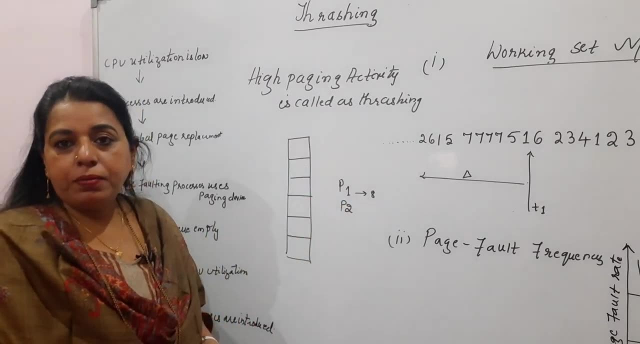 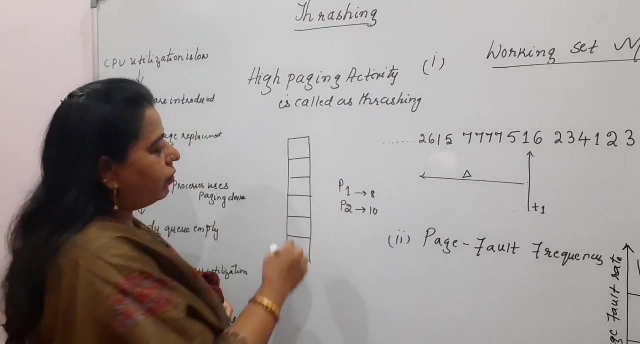 because only two pages are there and those two pages can be brought in whenever it is needed by the CPU for execution. Suppose, in the main memory, another process: get loaded p2.. Now p2 also needs some pages. So let us take p2 is having some totally 10 pages Now. what will happen? now? the 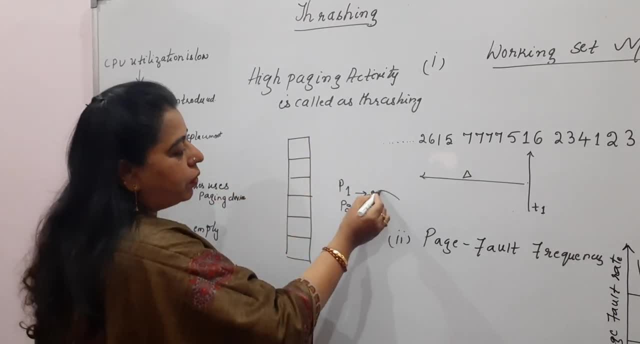 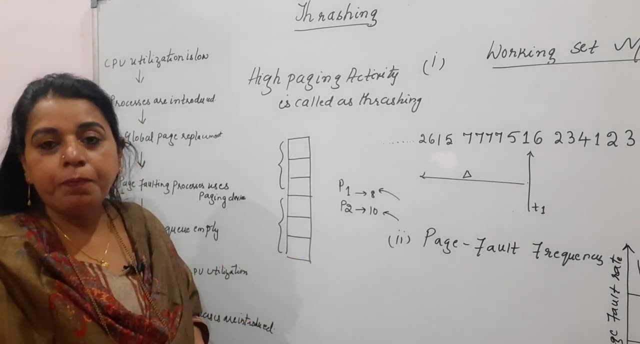 complete number of frames that are there. few frames will go to p1, few frames will go to p2.. So let us take: okay, p1 got some three frames, p2 also got some three frames. Later there will be some page fault happening for p2 because you can see now p2 is having 10 totally. 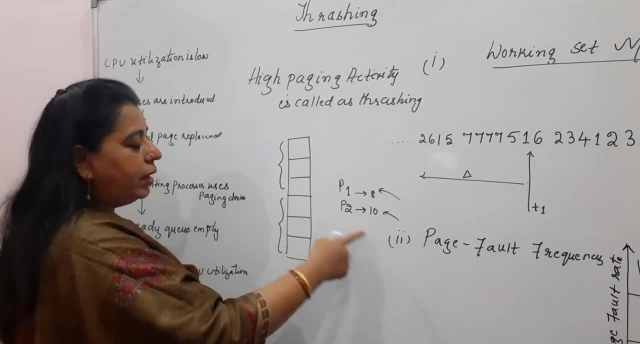 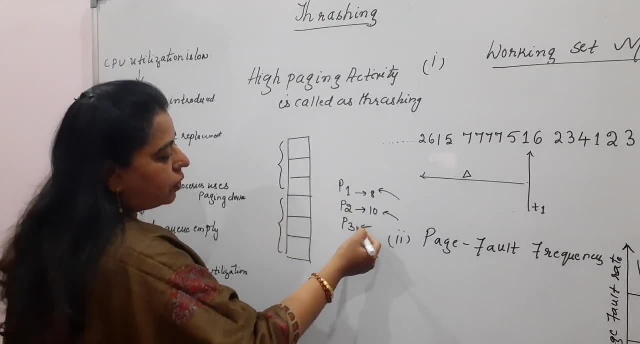 10 pages. So only three frames are given for p2, definitely page fault will happen. Now let us assume that there is one more process that is getting loaded and that process is also having some pages. Let us take six, then once again, what will happen? now this realloc, the frames will be. 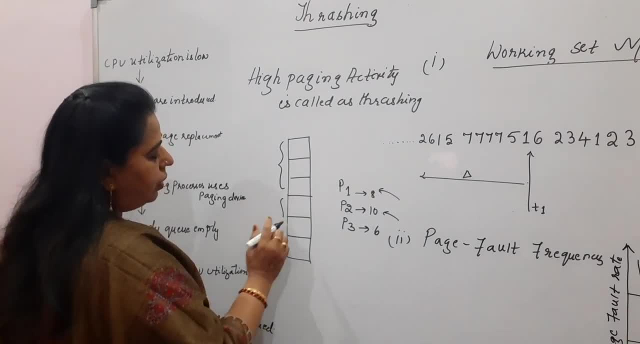 allotted to p3 also. Now let us take p3 also got some two pages. then p2 got two pages, sorry, two frames. So let us take p2 and let us assume that p2 is having some pages. So let us assume that p2 is. 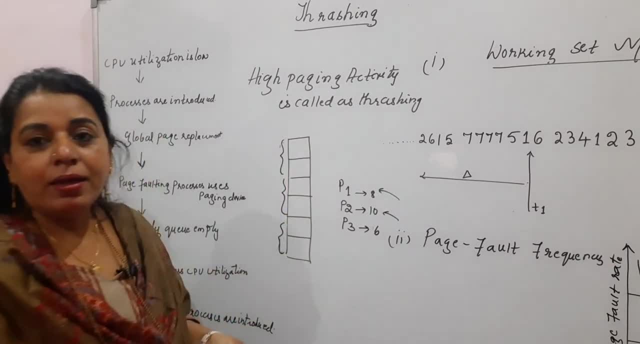 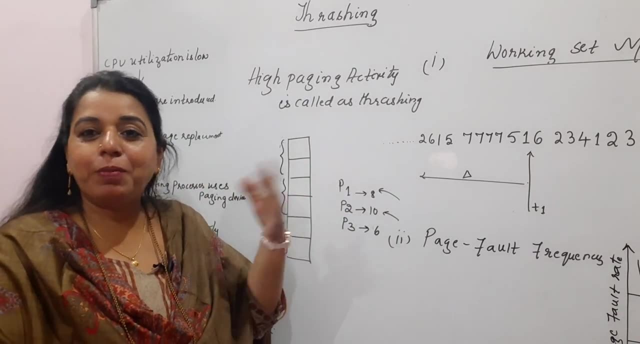 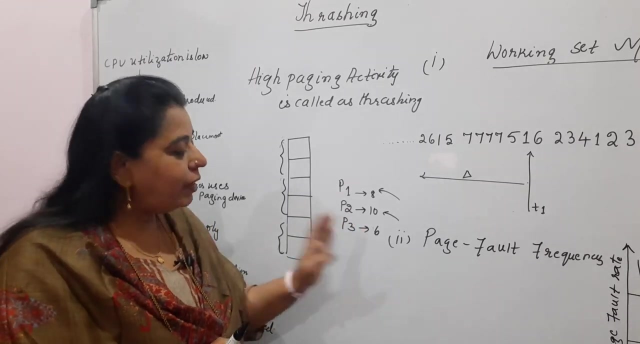 and p1 also got two frames. so this way the page, the frames, are what given to the different processes. but what you have observed is: initially p1 was very happy because p1 got all the frames in the memory for itself. later, when p2 came, few of the frames got allotted to p2 and later p3 came, then once again few of the 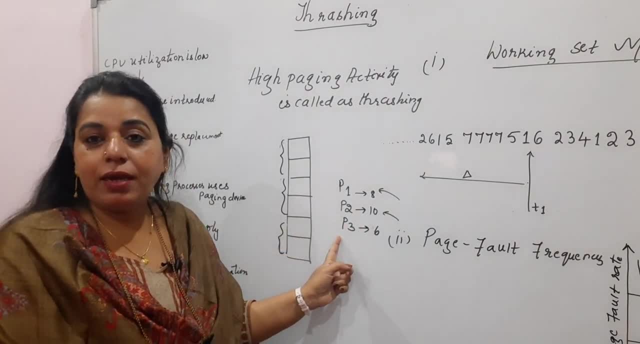 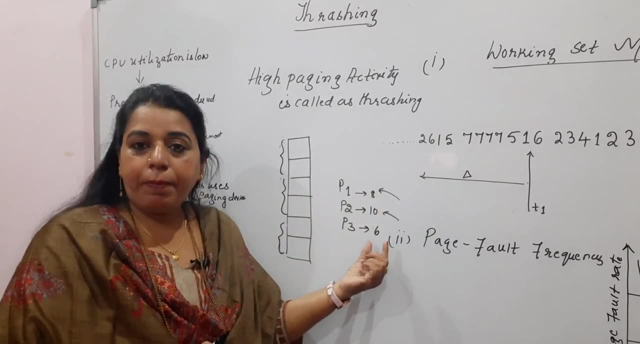 frames got. but what you have observing is all these three processes are processors will be experiencing what page faults frequently because they have got less number of frames but they're, comparatively, their pages are more. so, as and when CPU is in need of page, then it page fault will happen and, moreover, 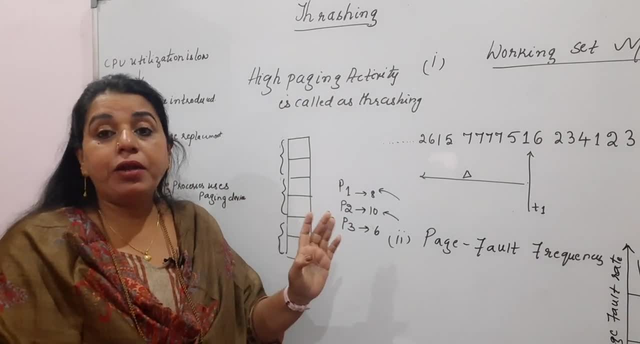 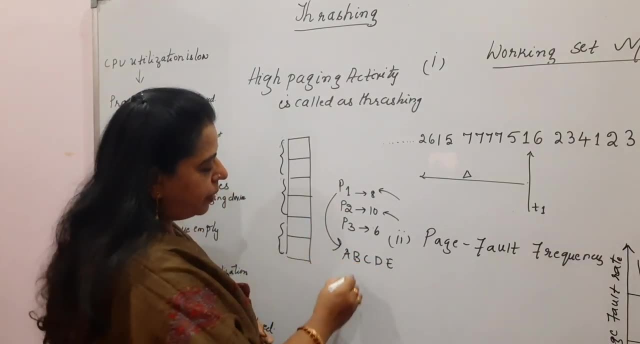 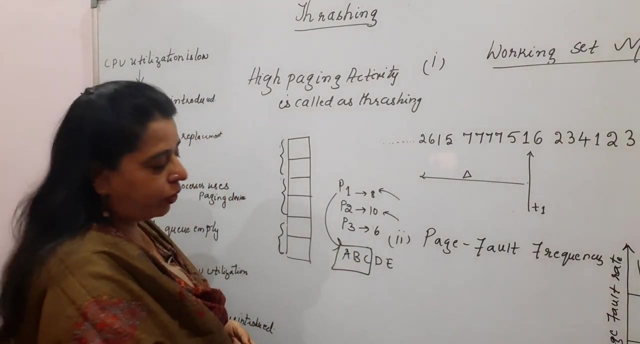 suppose if all these pages are active pages, active pages is what, like some PA, p1 is having some ABCDE. okay, active pages are there. at time being, you can assume that only three pages of p1 are there in the memory. D and E are in the 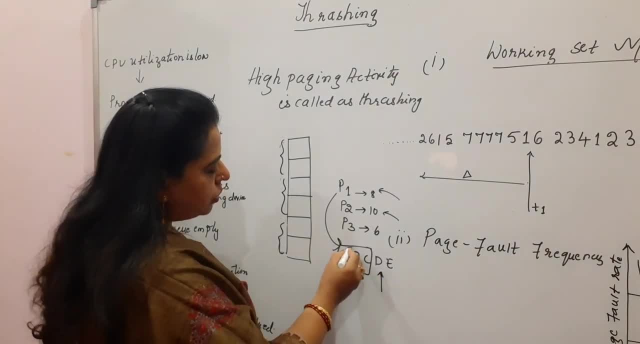 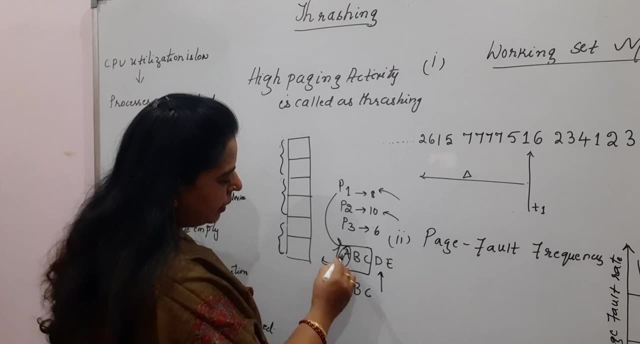 hard disk. so, but if you is in need of D, so they will take out A and place it. what place the D? D here in place of A? and what has happened is A is now in the secondary memory, but immediately CPU is demanding again a, a which was just taken out from the main. 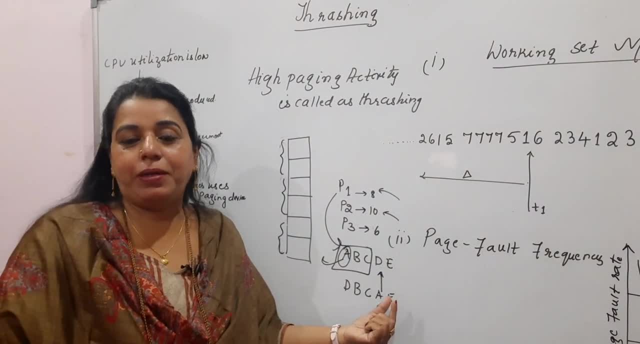 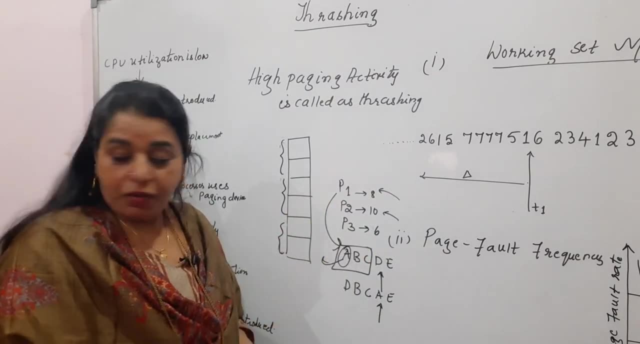 memory is once again in need. so we said those pages are called as active pages. so if all the pages of the processes are active, then page fault will frequently happen there, if at all. you want to have a plot of CPU utilization versus multi-programming, The graph will appear in this manner: 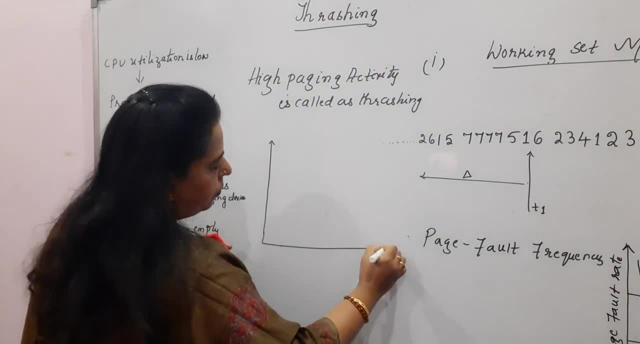 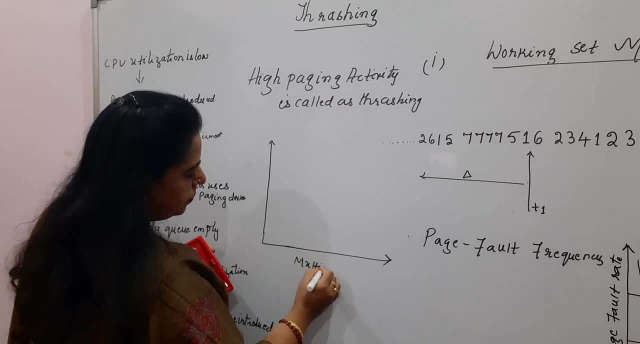 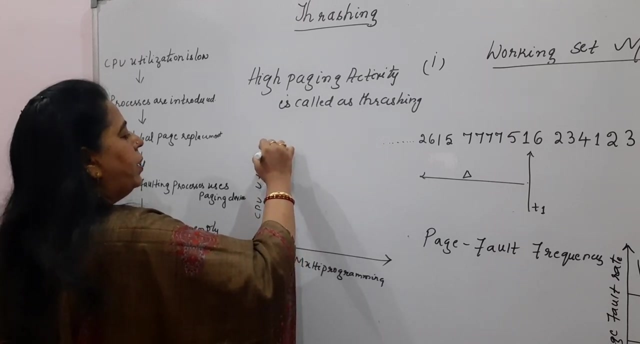 See, I can show you with a graph You put what the on the x-axis you can write down what multi-programming, degree of multi-programming, and on the y-axis you can write down CPU utilization. What do you mean by degree of multi-programming? The number of programs. 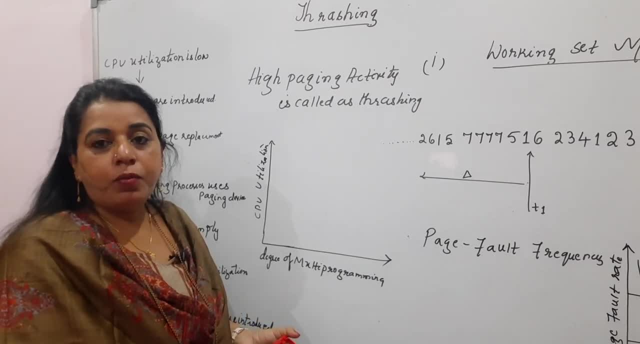 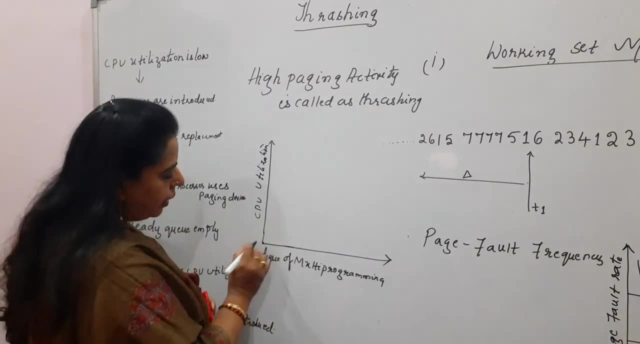 that are there in the main memory for execution. So if more number of programs are there in the main memory, then we said there is a high value for the degree of programming. Let us assume that degree of programming initially is here. That means just one process. is there One process? 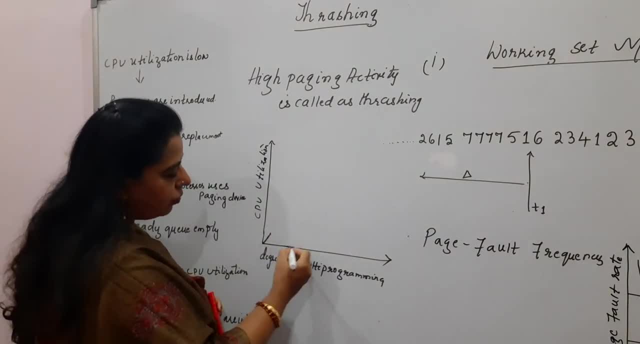 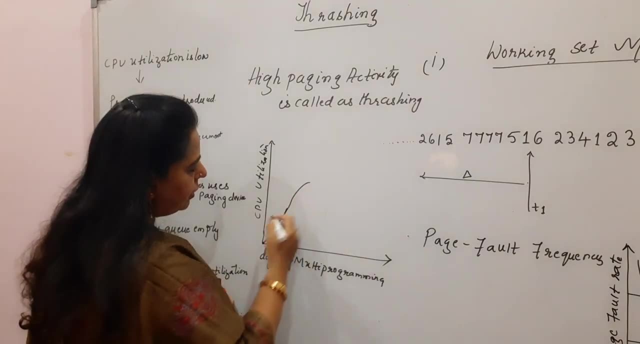 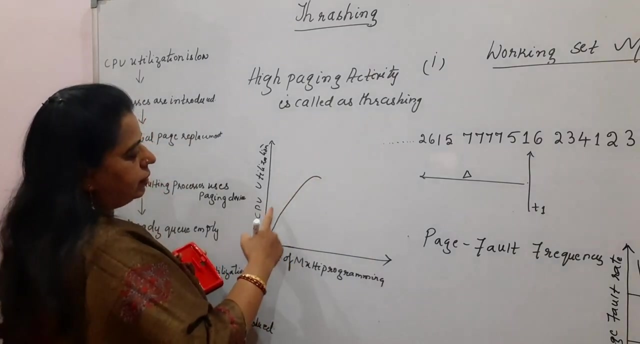 is there. CPU is what executing that process. As and when the number of programs get increased, then CPU will also what its utilization, The utilization, will also get increased. You can look here in this manner: the graph: the utilization for the CPU will also get increased. Now, at one particular stage, what? 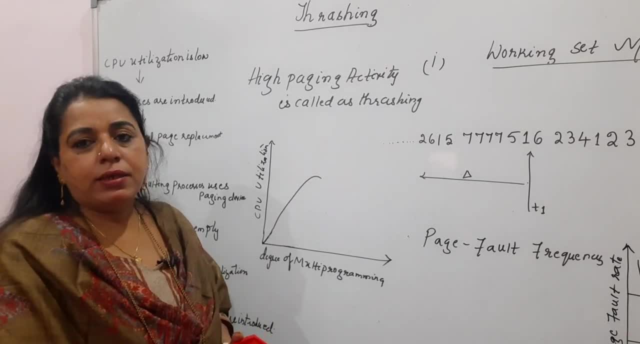 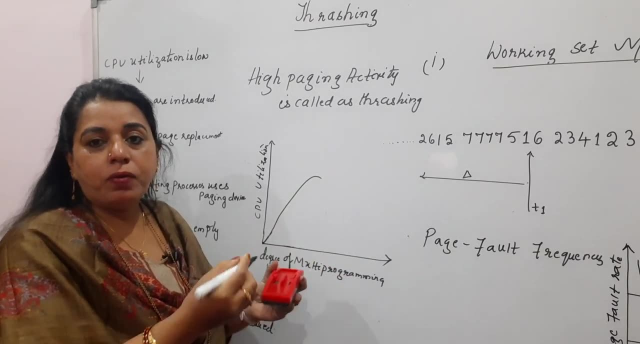 will happen, know. number of page faults increases like tremendously. number of page faults happen. Then what is happening? the pages are swapped in, swapped out. swapped in, swapped out. the system is completely spending the entire time for what to swap in and swap out. What about? 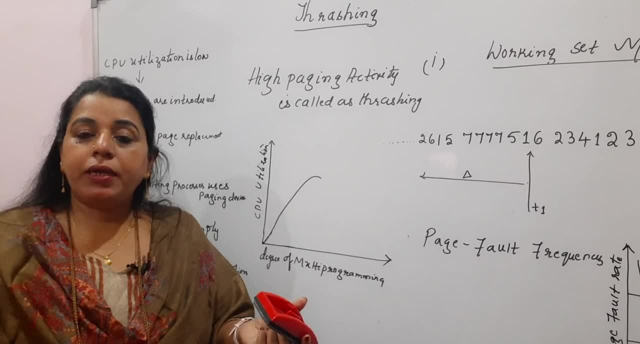 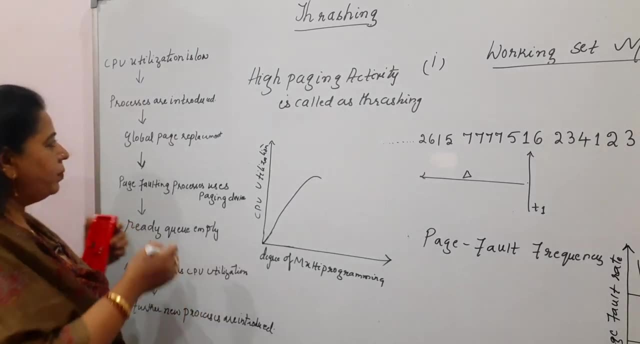 CPU utilization. CPU is not having any task to execute. the CPU is not having any process to execute because all these processes are queued up to the paging device. Look here. one more thing I can tell you is: see in this manner, if you look here as and. 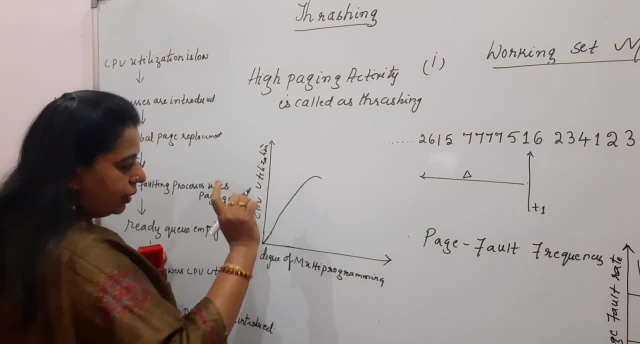 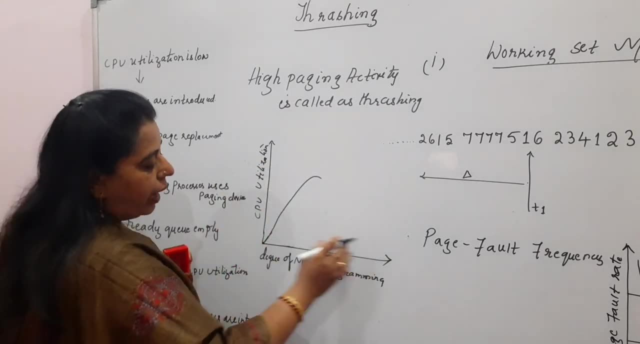 when the degree of multi-programming increases, the CPU utilization is increasing. That we can clearly understand and it has to happen. also, CPU is executing all these processes, But after certain time, as and when you increase number of programs in the main memory, the 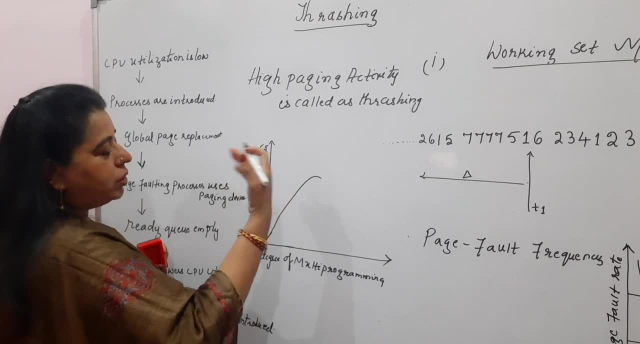 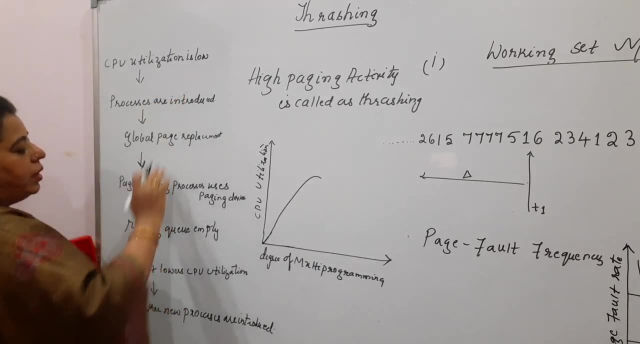 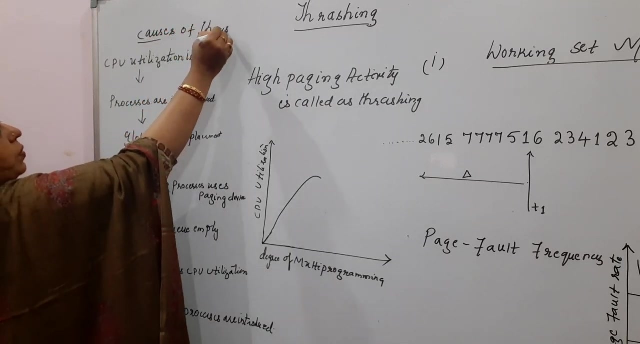 CPU is not having what the job of executing those processes, because all these processes are queued up for the paging device. You can look here: this is what is the cause of thrashing. causes of thrashing I have written here in a flow. okay, first, CPU utilization is low because what has happened? 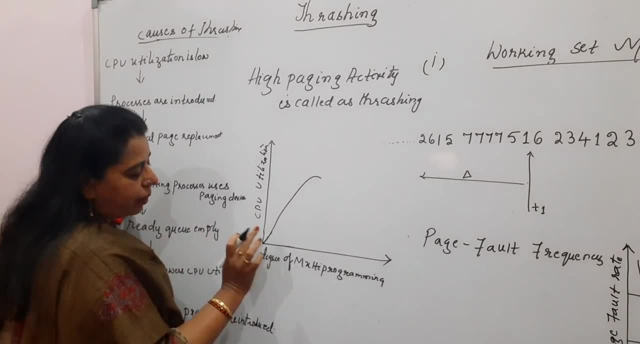 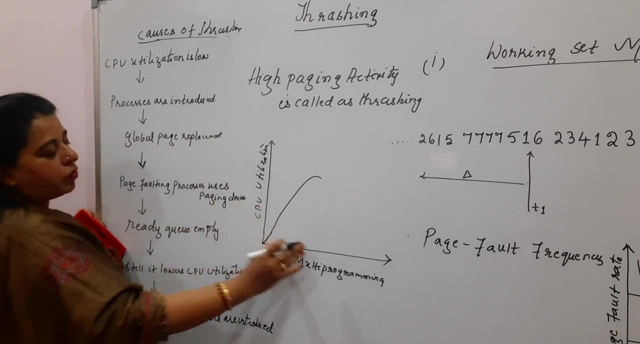 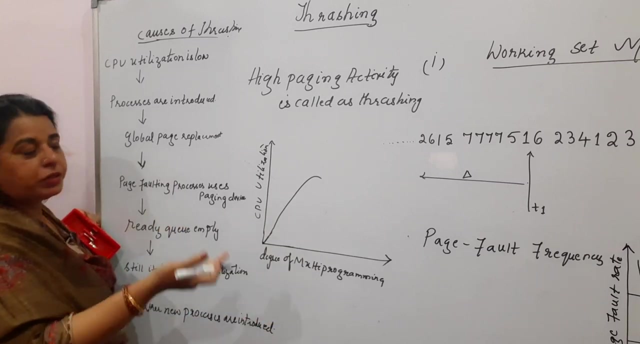 now. first, initially we made only one process to come over here in the main memory. then CPU utilization is only up till here. To increase that, what we introduced- more number of processes- then we are using the global page replacement. If you increase more number of processes, definitely what will happen? page fault will. 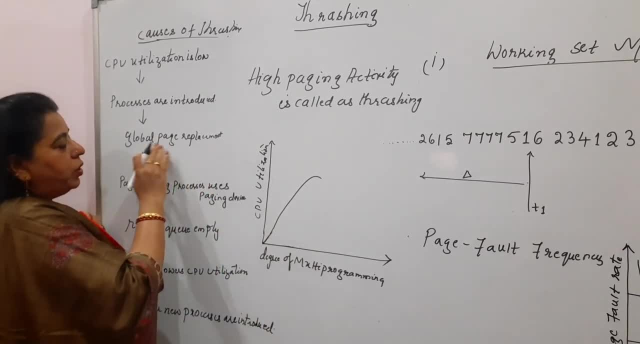 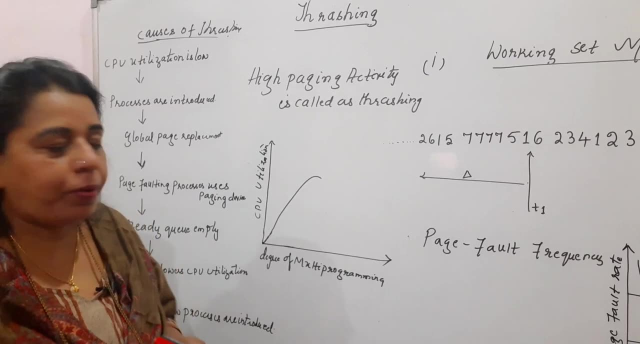 also increases, Then you have to replace the page. You are making use of global page replacement algorithm, wherein global is what a process can use the frames that are allocated to any other process also. Then what will happen? page faulting processes uses paging device. 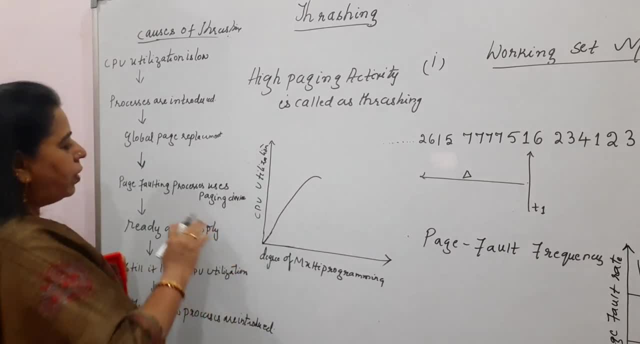 Because of increase in the rapid increase in the page Page fault. all these processes are queued up for the paging device. Then ready queue is empty. Definitely processes get executed if they are placed in the ready queue. CPU will execute those processes that are there in the ready queue. 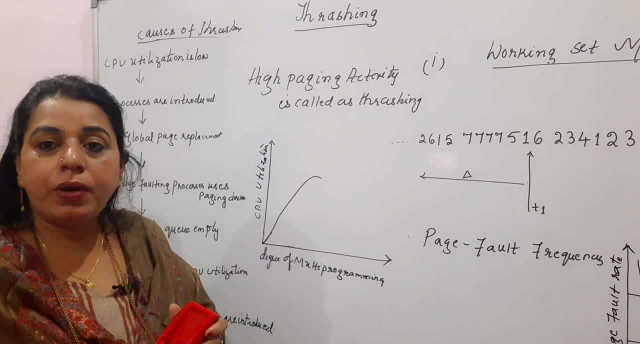 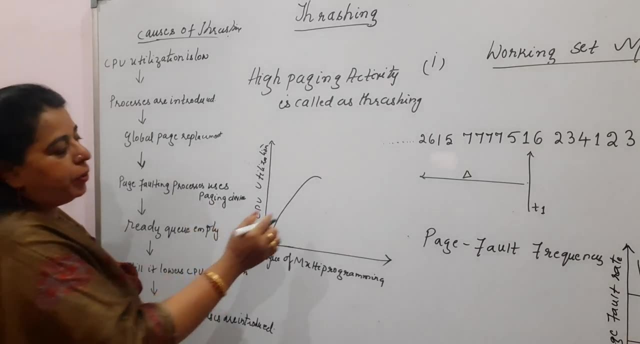 But the ready queue itself is empty, because all the processes are queued up for the paging device, because for all the processes the page fault has happened. Then what will happen? it will lower the CPU utilization. It will lower the CPU utilization. okay, Like this, you can show the graph further. once the CPU utilization is lowered, the system.